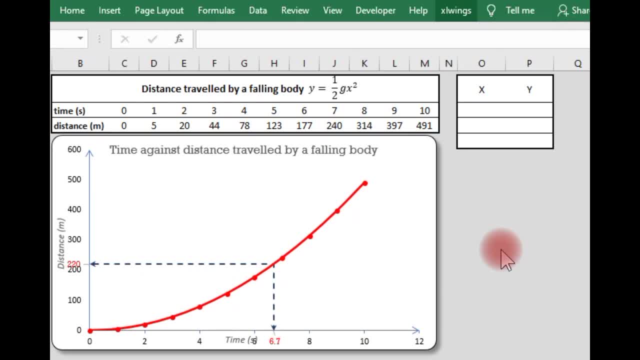 hello and welcome to another tutorial. in this tutorial, we are going to be looking at how to trace or project values on a graph, and that's what I mean by this. this curve shows the distance traveled by a free-falling body at any point in time, so we want to be able to trace on a graph that, at 6.7 seconds, the 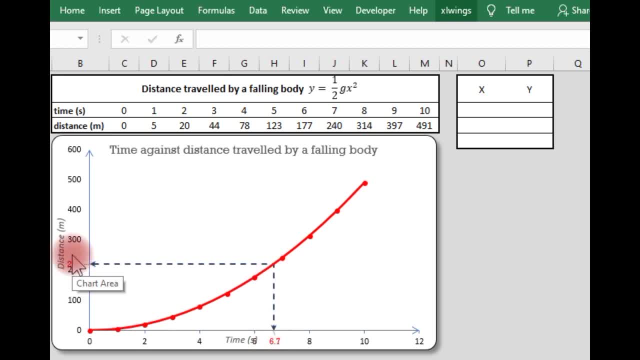 body will have traveled 220 meters. and there's the formula. well, y being the distance is related to half of gravity times X, which is the seconds squared. okay, so let's not talk much. let me just show you how to do that. okay, so let's remove everything left with only our graph, and then we can begin. 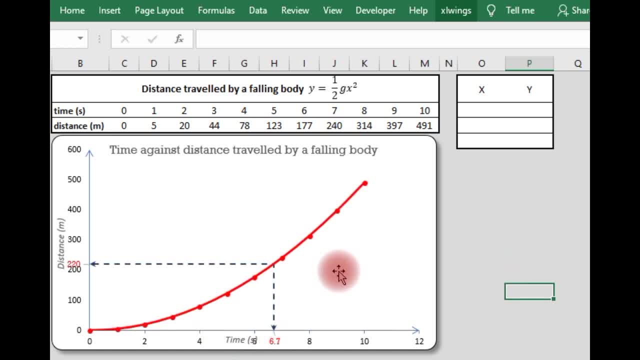 okay, so from here, basically, what we have done is that there's a line from this point to this point and there's a line from this point to this point. so we have point one, point two, point three, and this point has been connected by a line that 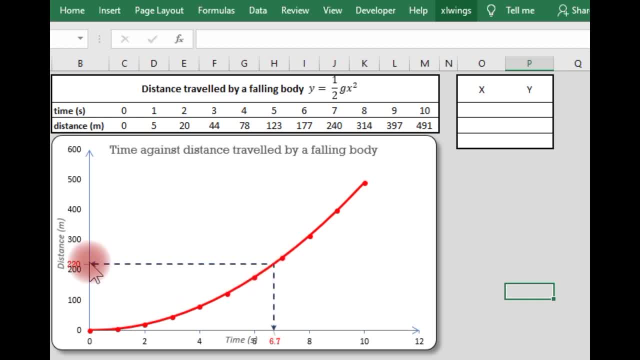 is basically what you've done. so let's note: this is 220. this is point seven one. so let's count back and just do the same thing. so we have our 220 here and our 6.7 here. so what it basically means is that we have a point here, which is when the y 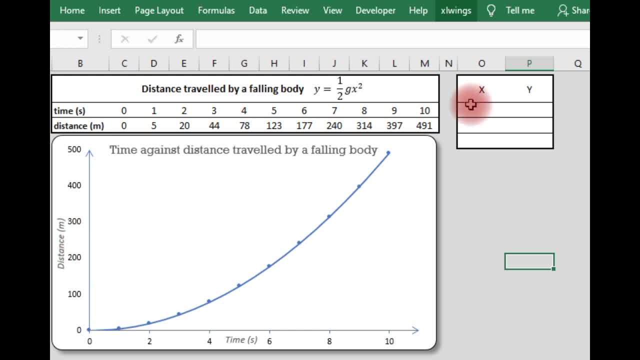 axis where x is zero and y is 220. so our x is zero and our y is 220. that is the first point. then it projects to a point here where our y is still 220, but our x is now 6.7. so our x will be 6.7 and our y will be 220. and then, finally, the third point. 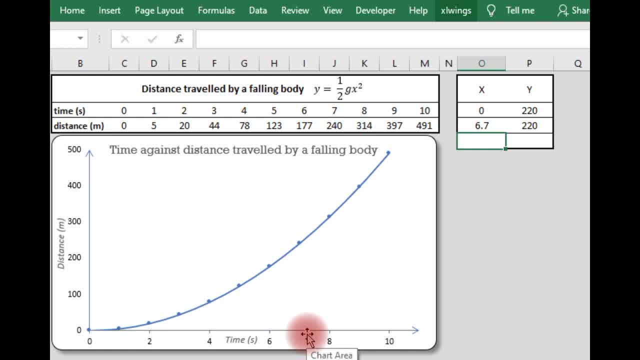 which is somewhere around this place where our x is 6.7, but because we are on the x axis, our y will be zero, so 6.7, and then our y will be zero. so now that we've done this, we are going to add it. 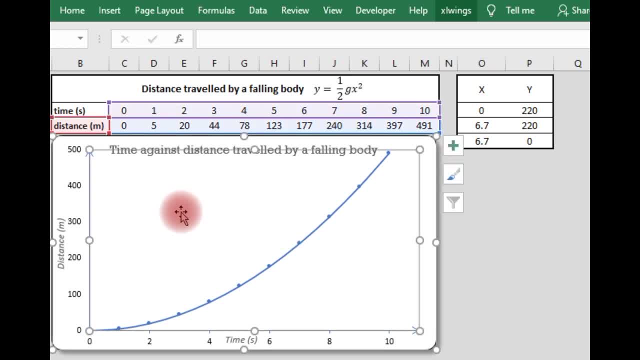 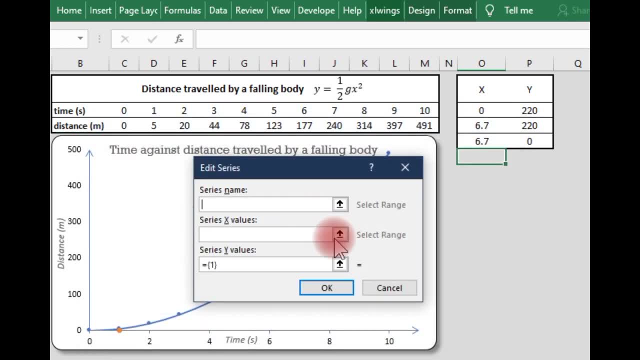 our graph as another line which will be drawn. so, to do that, we just do this, select data- and then we say add. so we are going to add another series. these are x values for the swiss name- you can leave it blank- and then these are our y values. okay, then, once you do that, you 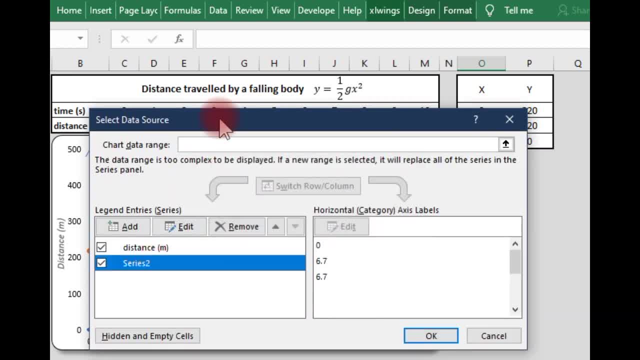 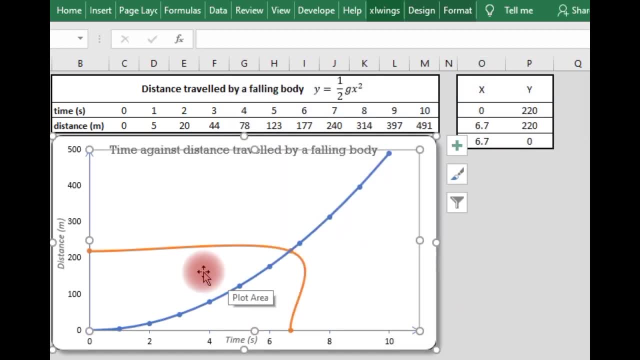 see: okay, let's move this up so that it will happen. then you see, okay, okay. so basically it is there, but it looks curved and we don't want it to be. can we want it to be street? so what we are going to do is we are going to come to the chat menu here. 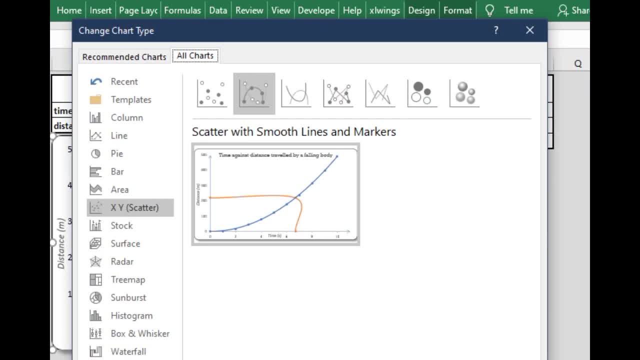 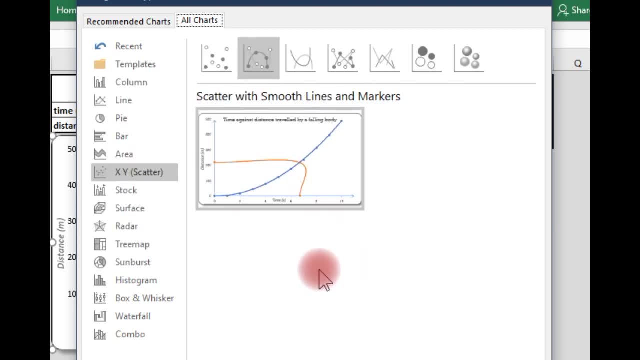 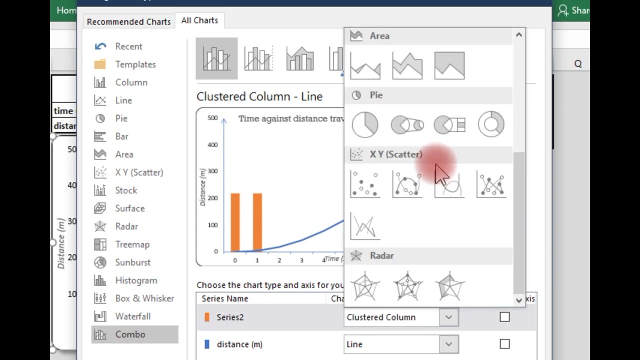 and we say: change chat type. what we are going to do is we are going to make it a combo chat. and that's how you make a combo chat. that means a chat with different elements. so you come to combo. for the first one, you make it scatter with smooth lines and then for the 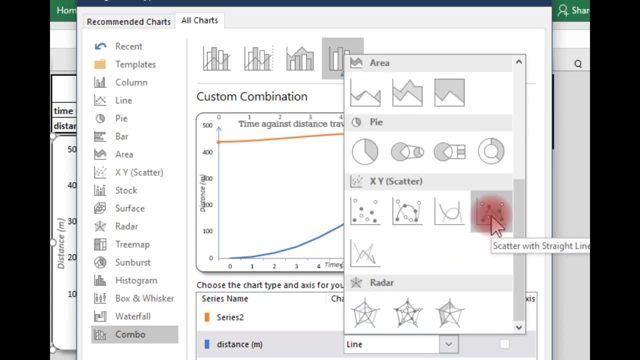 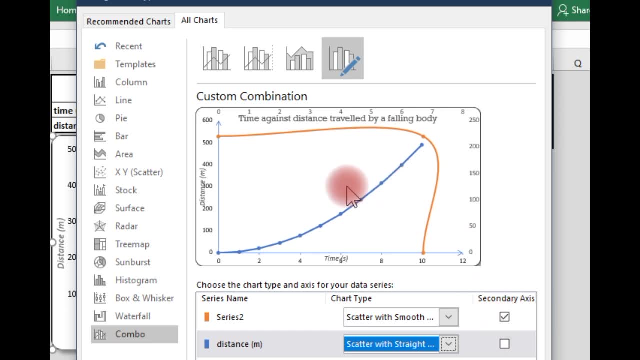 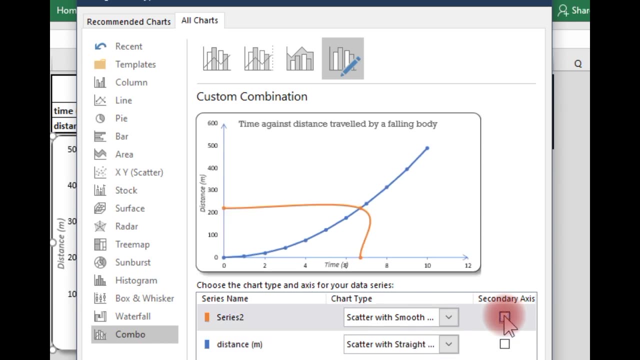 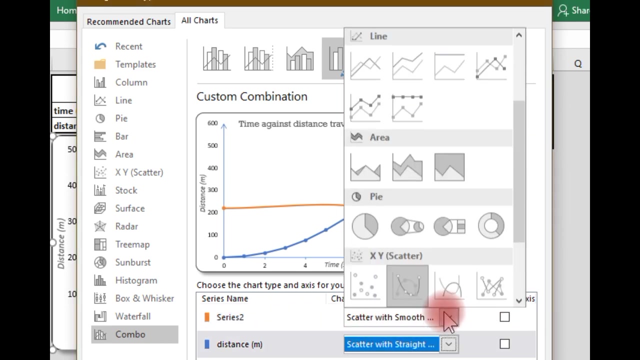 second one: you make it scatter with streets, lines, street lines, and Marcus, yeah, choose, select that one. and then what is still causing this confusion is that this one has been put on the secondary asus. she move it, remove it so that they are all on the same asus and then, sorry, our, our series 2 is rather 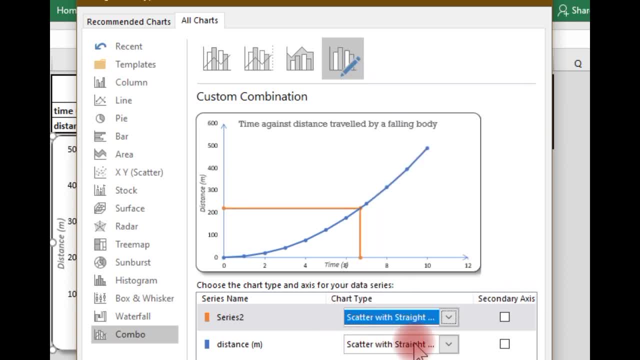 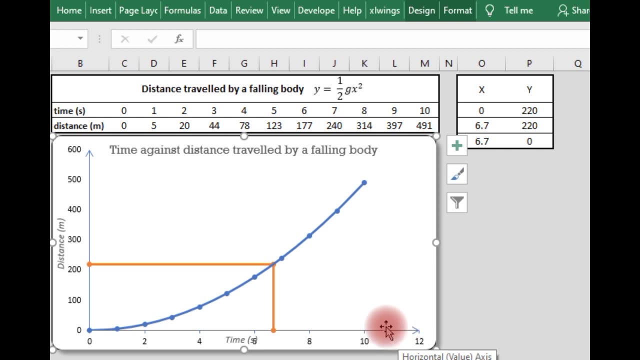 the one that should have street lines, and then our sheets, like, should be scattered with smooth lines. you want a cave. and then, once you've done all this, we see, okay, and that is it, we get our graph. but this, since this one is the one that is being used to crease, we don't want it to. 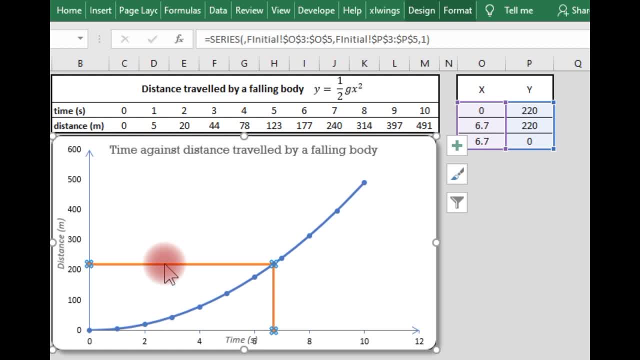 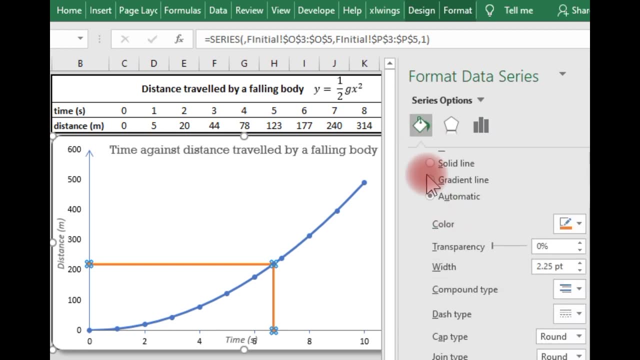 be very bold. we don't want it to take all over, to take over the whole graph, so we turn it down a bit, right click and see format, the data series, and then we come here, change some of these options. so let's make it black and then let's. 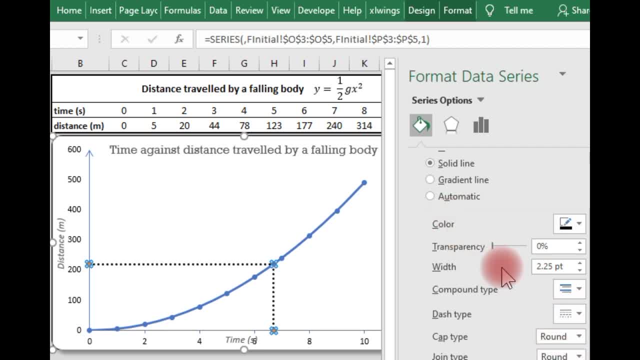 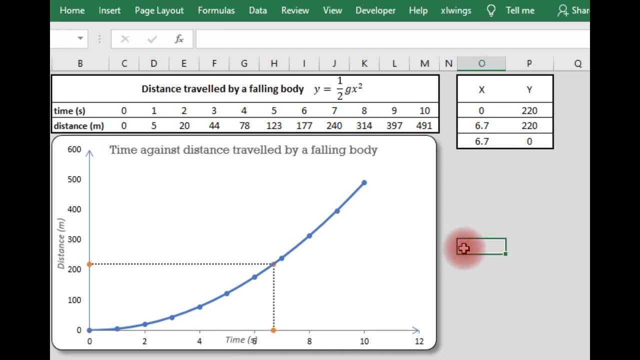 change the dots, let's reduce the width. okay, this visible now we can change that, you know. once you've done that, we are okay. the problem is when this currency is that we have our s values and our y values being hard-coded, we actually pick them from a. 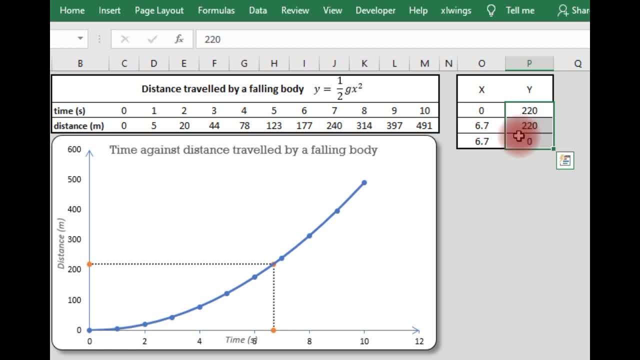 bunch of values or � and then we just switch to the opposite side so we got a lot of values so we change the value one to 3 and make sure to notice that there are all the values that we need to base it on exactly I sugarہ shut out 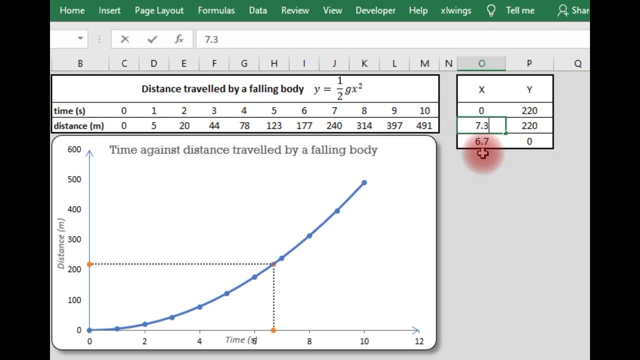 our way to that. we've already done so what happens if we want to look at baby 7.3 or any? if you got a light, what will happen is: should i, if I think this to 7.3 s 1147.3al gerade? 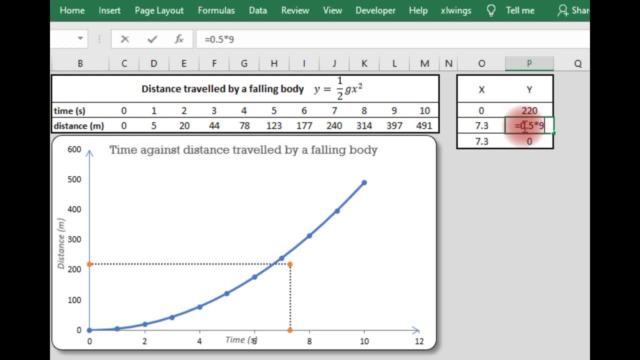 thing. so let's put the formula and then reach to the power 2: okay, so that is it. and then let's make this figure, let's make it equal to this one, so that soon as that one changes that out to change, and then let's make this figure to equal. 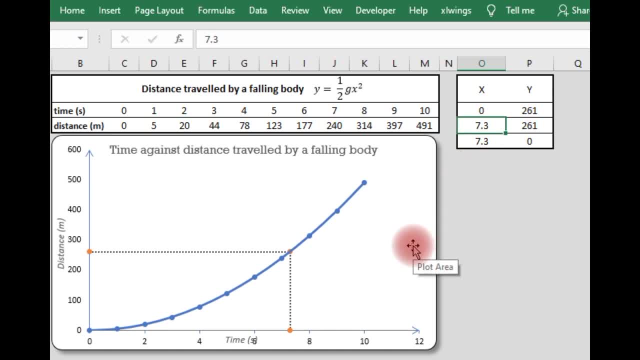 to this figure, and that is it. anytime we change one the other, which, so let's look at 9.3 and immediately our graph will move to 9.3. okay, so this is the first method of doing it. if you have any questions, leave them in the comments. you. 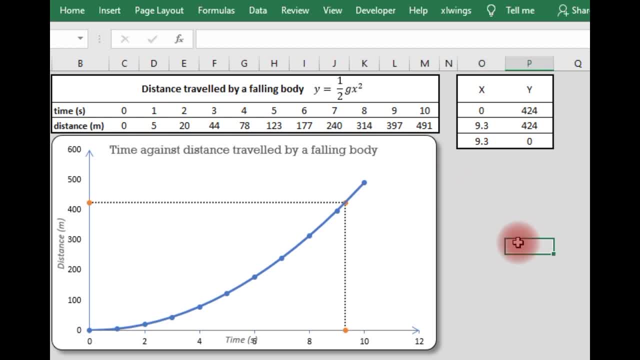 can also reach me on whatsapp, if you have my number or anything, and I'll get back to you. so this is basically how to do it, and one of these tutorials I'll teach you how to make nice graphs like this and how to format your work to look nice. okay, so let's end this. catch you another time for the second. 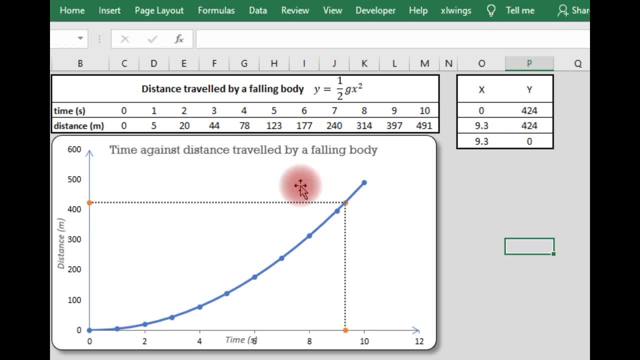 tutorial which I'll show you the second way to do something like this. thank you.